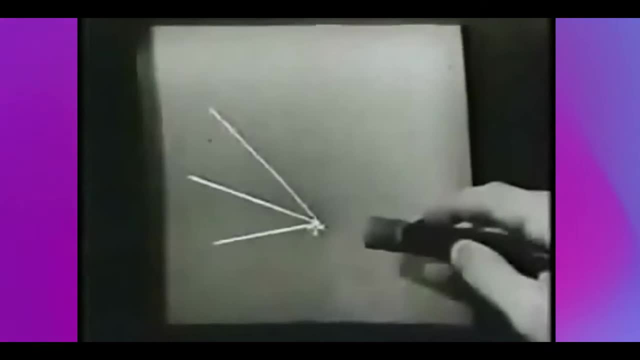 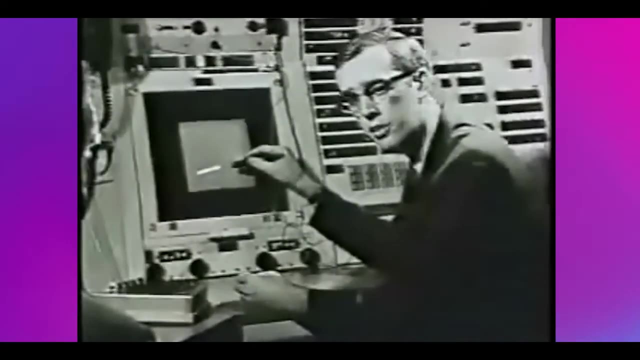 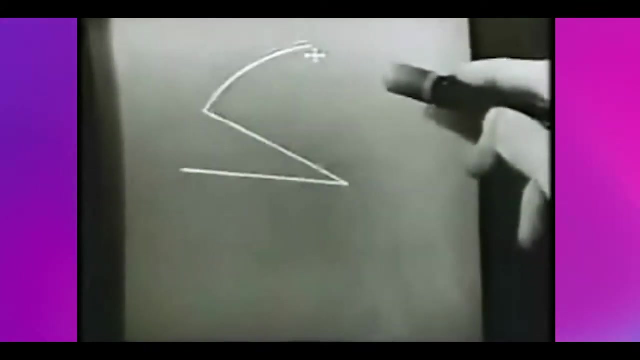 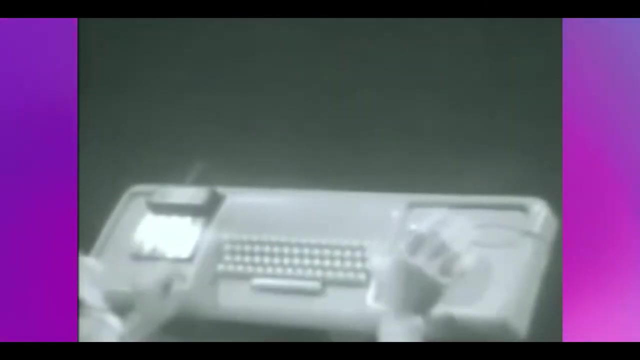 grandfather of drawing tablets of today's date. Sketchpad uses drawings as a communication medium for the computer. It sketches directly on a computer display with a light pen. The information sketched can include straight-line segments and circle arcs. The following year, 1964, the first computer mouse was invented by Engelbart The mouse. 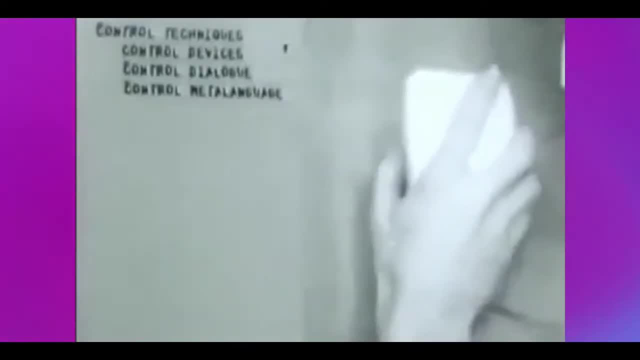 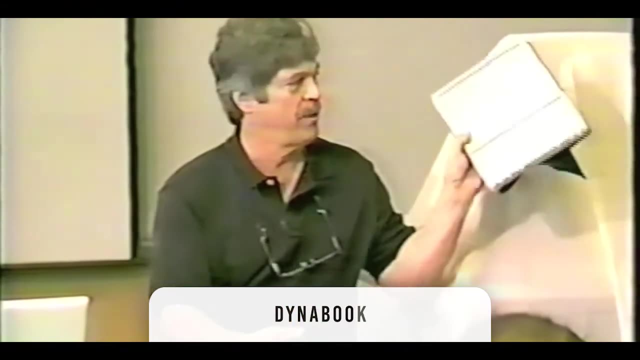 as early models, is used to interact with the computer through a cursor in the screen. The mouse movements and inputs are also used to interact with the computer. Dynabook, Alan Kay's vision of a personal computer, is described as a thin, portable device. This 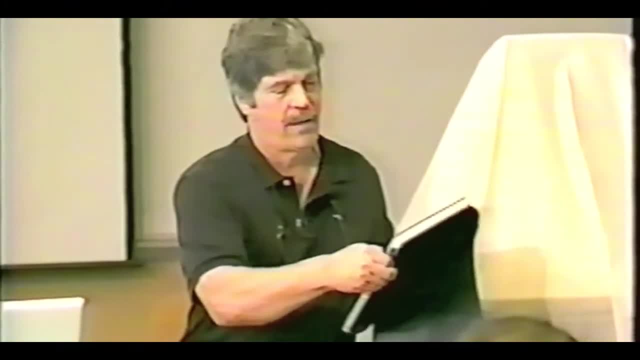 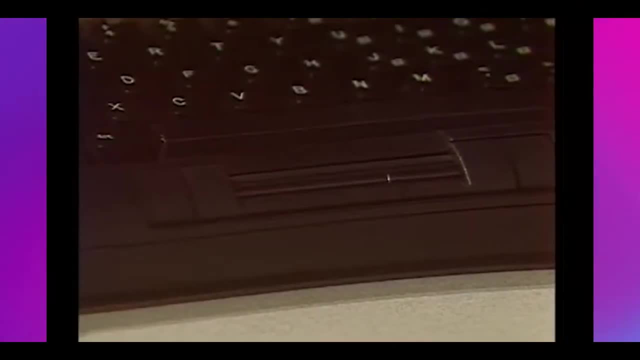 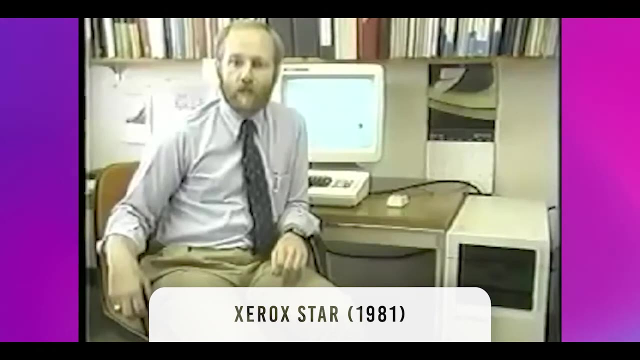 concept was created, way advanced than the technology of its time. The first portable personal computer was the Grid Compass 1101, designed by Bill Moggett in 1980, 11 years after Alan Kay's vision Xerox Star. Xerox Star was released in 1981. It had a mouse-driven. 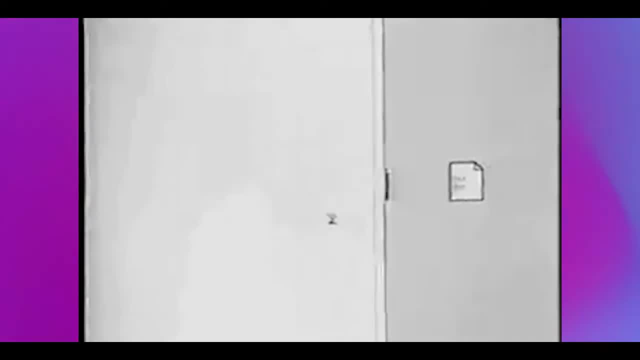 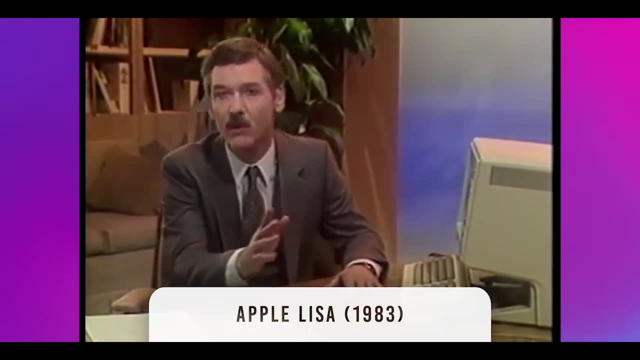 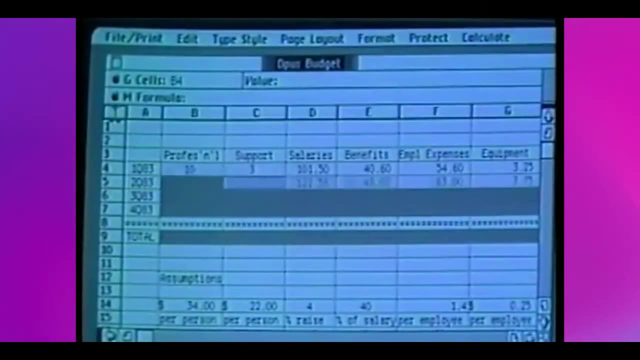 graphical user interface, built-in Ethernet networking protocol and optional laser printer. This was considered far ahead of its time. Apple Lisa- Apple Lisa is a desktop computer developed by Apple, released on January 19, 1983.. It is one of the first personal computers to present a graphical user interface in a machine. 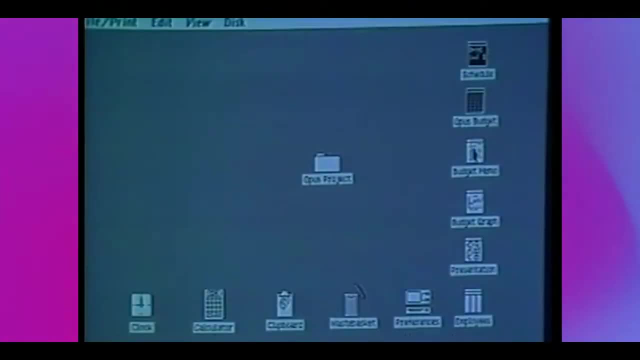 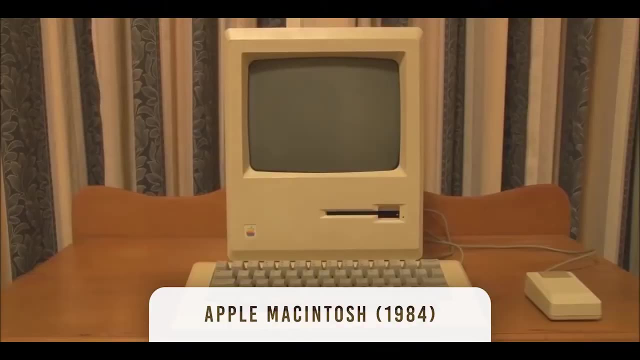 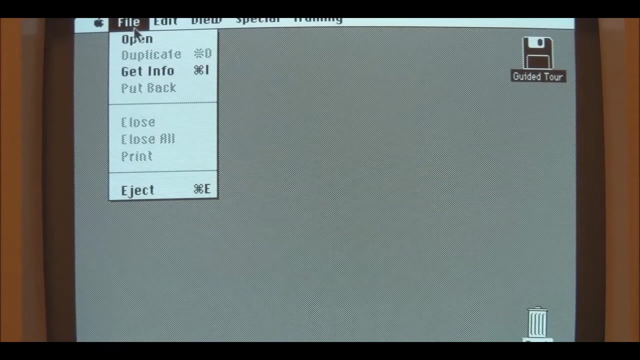 aimed at the individual business users. It offered a document-centered graphical interface based on the metaphor of desktop, with icons, folders and trash bins. Apple Macintosh. Apple Macintosh is a line of computers introduced by Apple Inc in 1984.. The Mac 128K had an 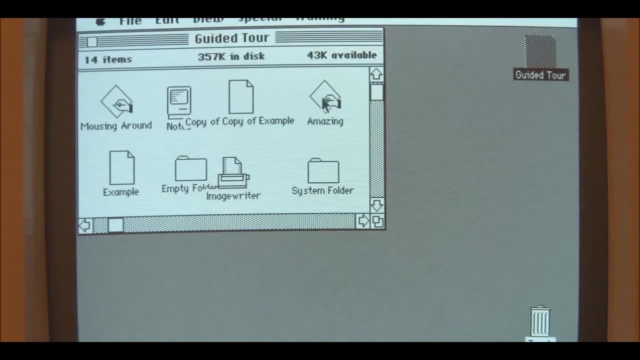 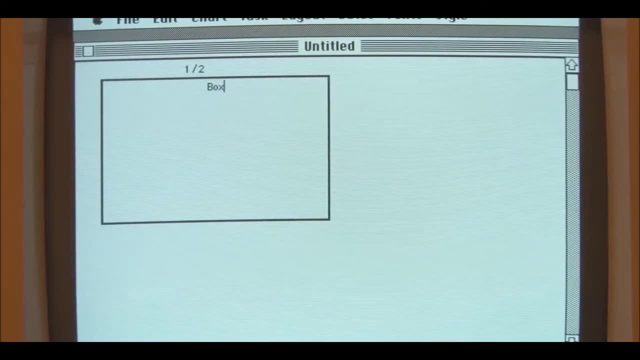 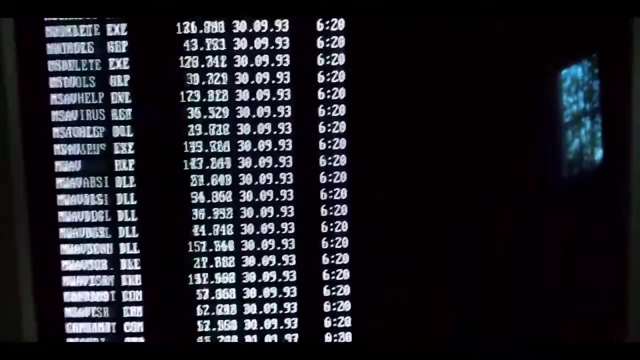 easy-to-use graphical user interface that utilized icons, windows and a mouse. Apple Macintosh are a much more advanced machine than the previous Apple Lisa at a cheaper price- MS-DOS- MS-DOS is a non-graphical operating system. This means that all commands given to the 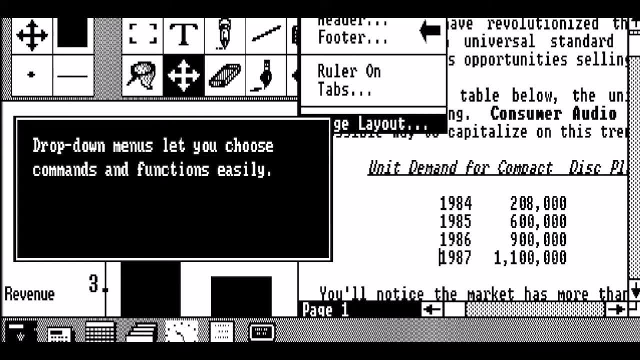 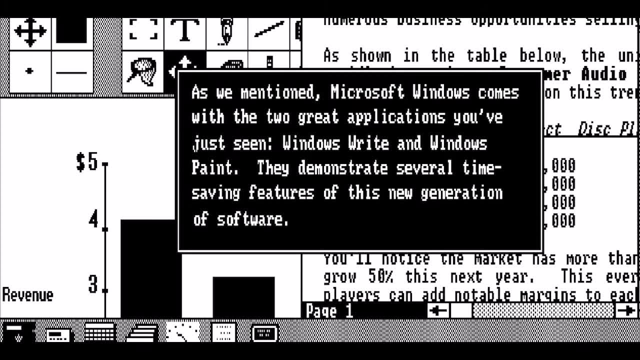 computer must be either typed in from the keyboard or entered from a file. It is a highly-useful tool. It allows the user to open, navigate and manipulate files on their computer from a command line instead of a GUI like Windows- Windows 3.0. Windows 3.0. Two years later, Microsoft released Windows 3.0. It came with a lot of improvement, but also with lack of multimedia and network features, which made Windows 3.0 replaced quickly by Windows 3.1, which is made fancier, provided multitasking support, improved programs and. 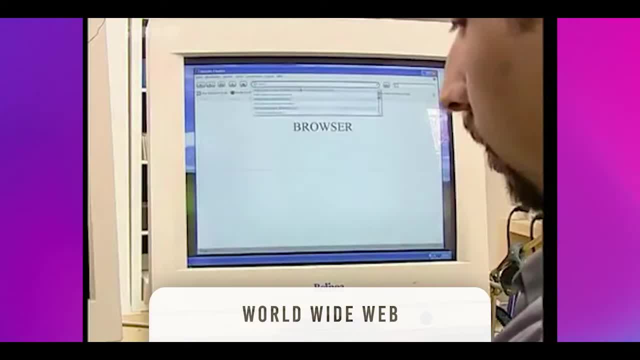 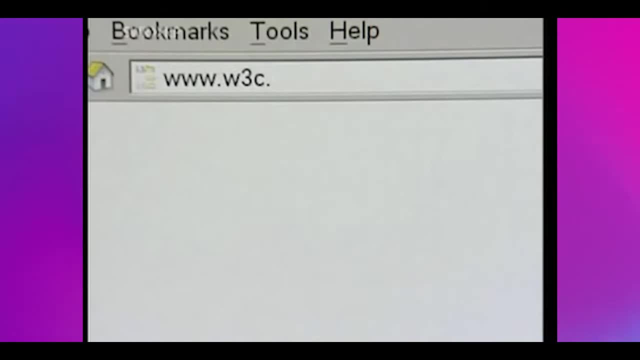 more advanced features. Windows 3.0 was designed to provide a Baseline of apps to Windows features. Within the same year, 1990, Tim Berners-Lee made an information management system, which then became the World Wide Web. It soon became the prevalent technology in internet. 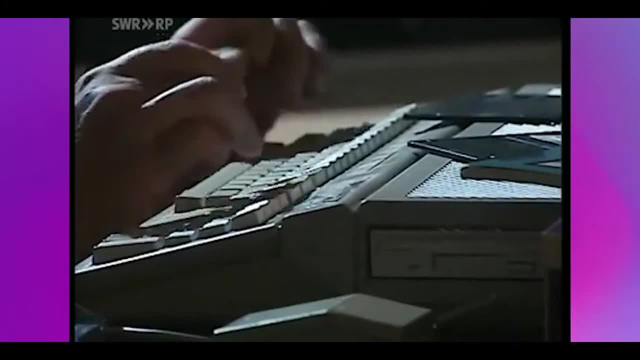 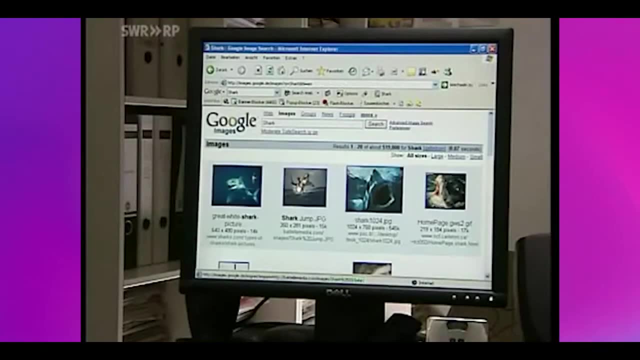 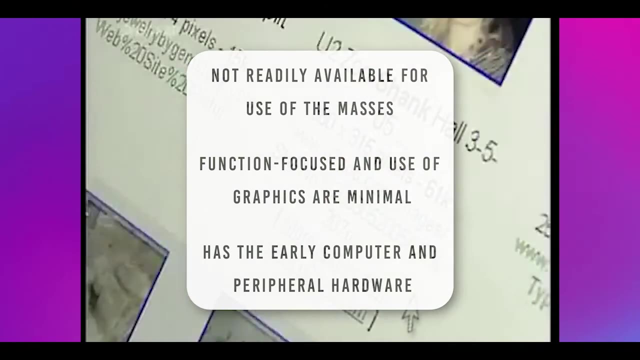 and a global information medium. in the 1990s, After the global launch of the World Wide Web, the world enters a new stage of technology In comparison from the past generation, which is not readily available for use of the masses, function focused and use of graphics are minimal. 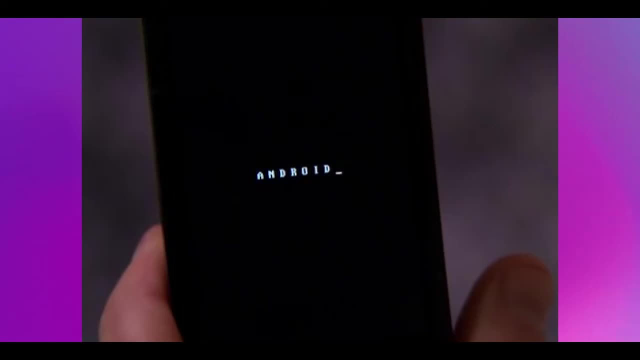 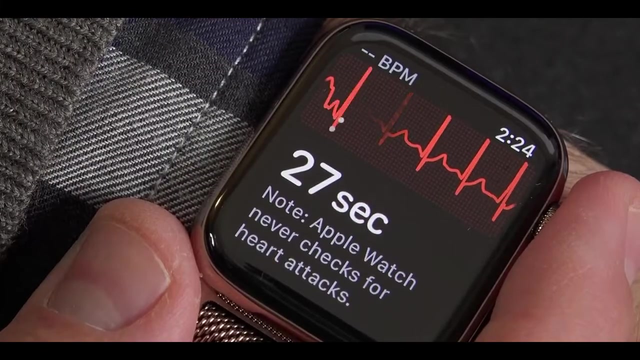 it has, the early computer and peripheral hardware At the start of the 20th century. new forms and innovations in technology and HCI are sprouting. Improvements in revisions are starting to happen more frequent than before. The very first iPhone was released in 2007.. 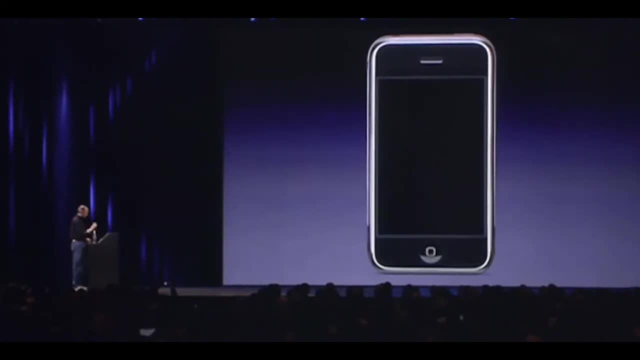 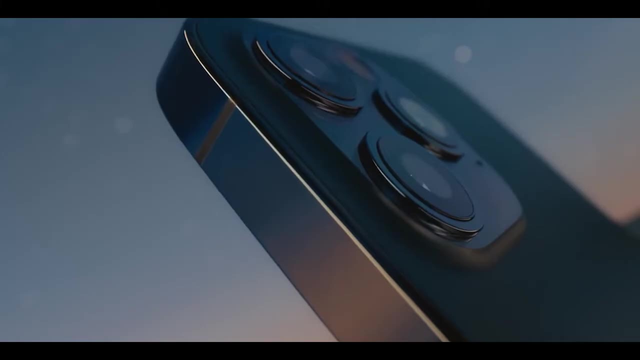 It featured a 3.5-inch display, which was considered as widescreen during its time. It has the features of a camera, iPod and computer-in-handheld device. The latest iPhone that was released boasts of much better specifications than those in the previous. 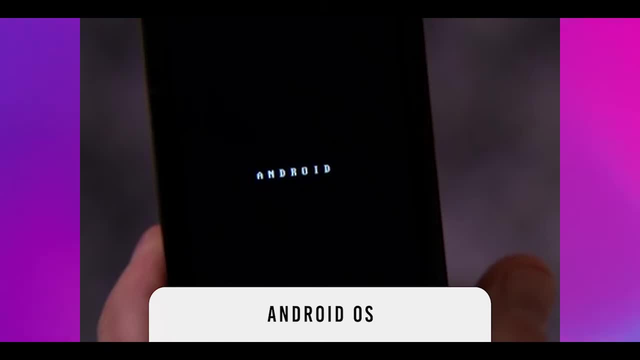 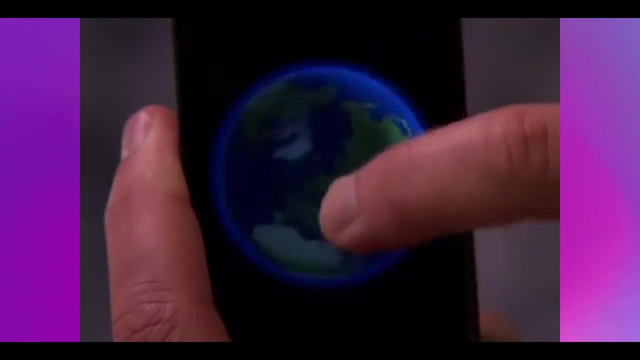 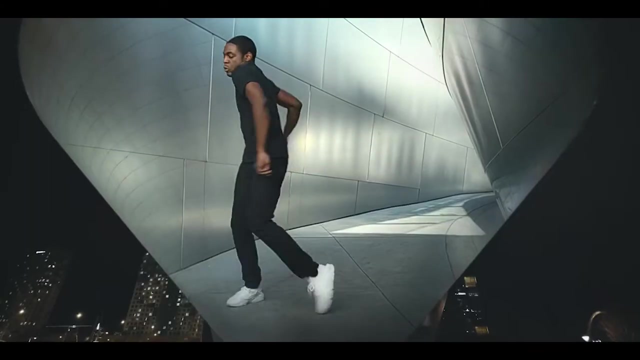 generation. On the other hand, the Android mobile operating system was developed by Google to be primarily used for touchscreen devices, cell phones and tablets. Just like the Apple's iPhones, Android operating phones and tablets are handheld devices that could take pictures, create and edit documents and media. 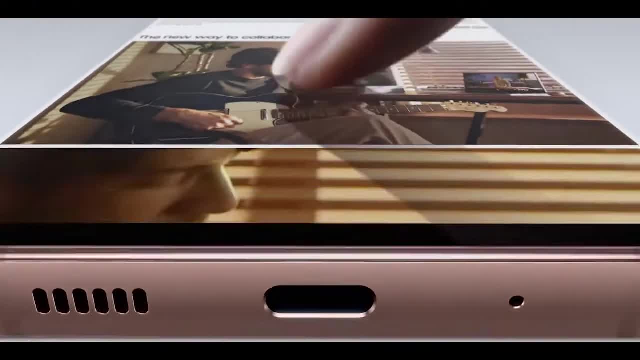 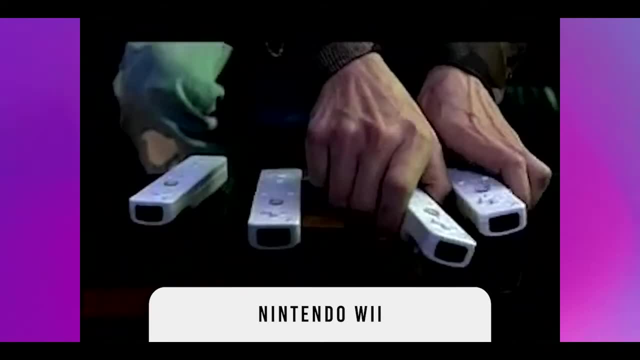 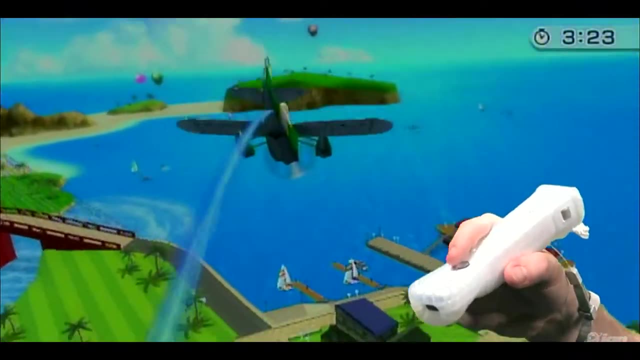 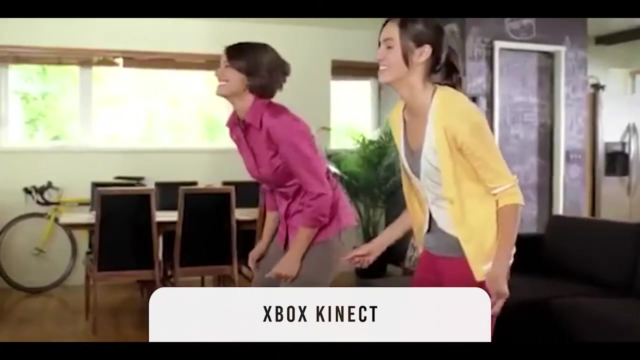 In 2006,, Nintendo released the Wii console with its famous Wii Remote Controller, a handheld pointing device that detects movement in three dimensions. It enables users to simulate real-world sports and activities through different games. This paved the way for game consoles like the. 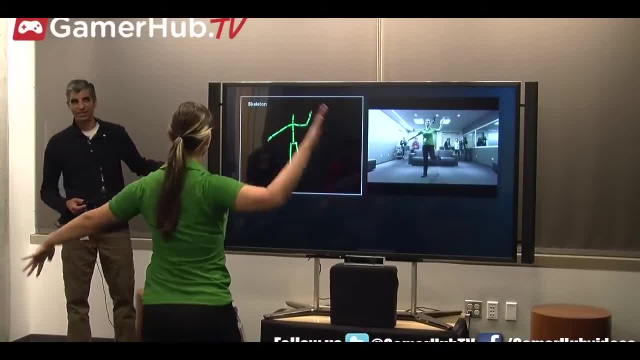 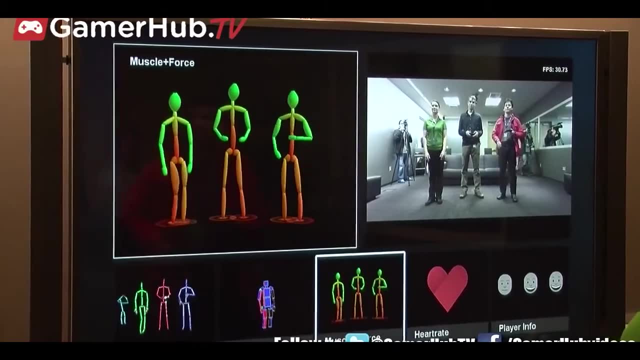 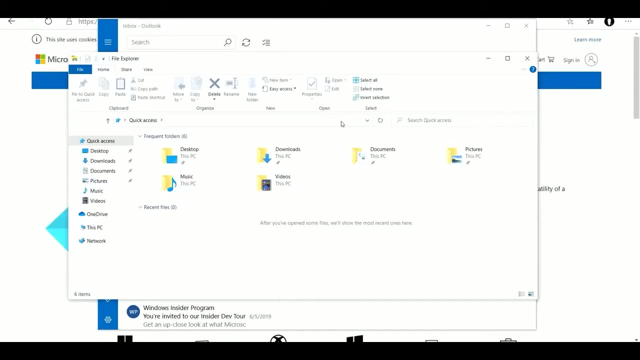 Xbox Kinect, a feature from Microsoft Xbox which uses the Wii Remote Controller to simulate real-world sports. The Wii Remote Controller uses depth and motion sensing technology as input for the console to recognize movement without a remote or controller. Windows 10 is a series of operating systems developed by Microsoft, released in 2015.. Windows 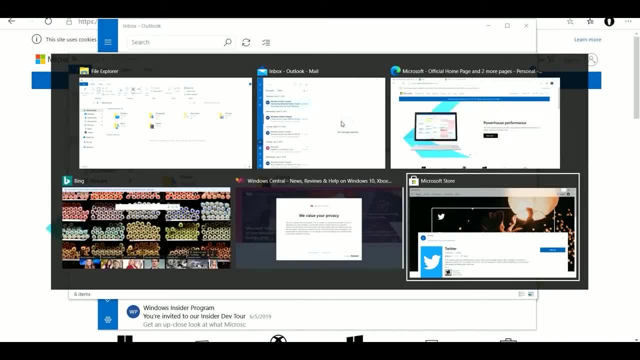 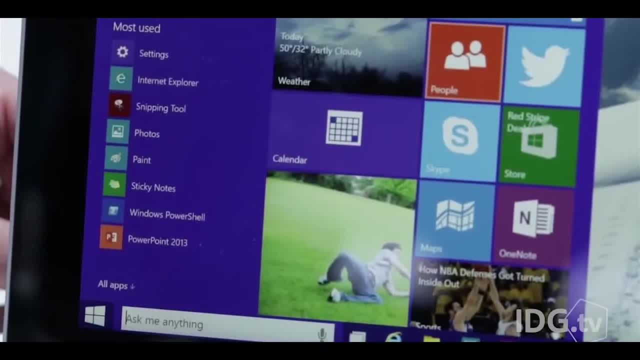 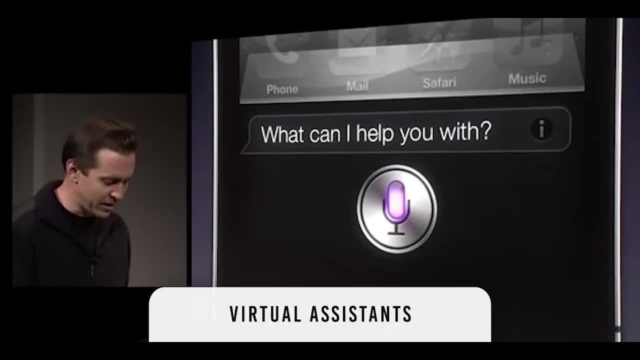 10 made user experience and functionality more consistent between different classes of device. With the rising popularity and availability of laptops, netbooks and computer systems, Microsoft made the Windows 10 adaptable into different systems. Another innovation in this era was the Intelligent Virtual Assistant, or Intelligent Personal. 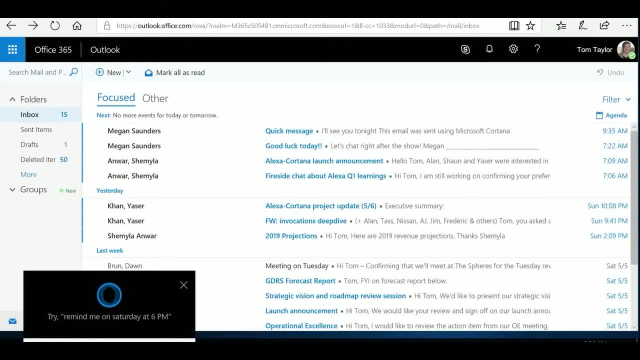 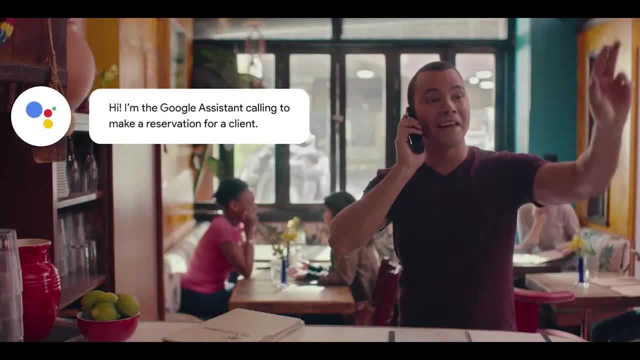 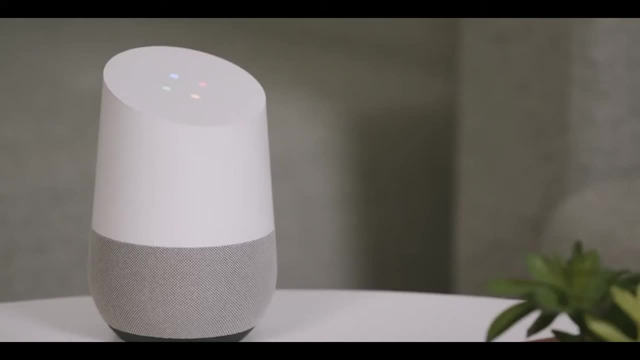 Assistant. It is a software agent that can perform tasks or services for an individual based on commands or questions. These virtual assistants can interpret human speech and respond via synthesized voices. Users can ask questions, control home automation devices and media playback via voice. Also manage other basic tasks such as email, email, e-mail and other basic tasks such as email, phone calls and other other important tasks. All of these devices are able to do the job of voice and control home automation devices. It is also possible to control home automation devices and media playback via voice. Also manage other basic tasks such as email. 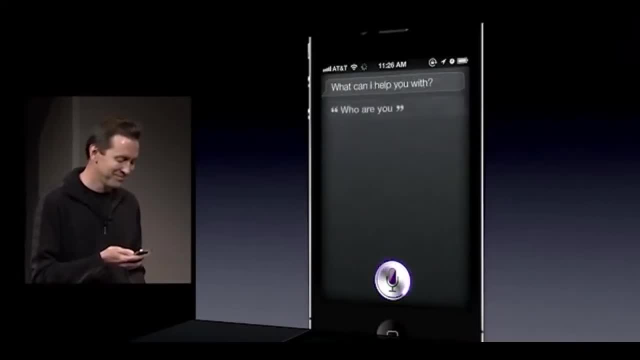 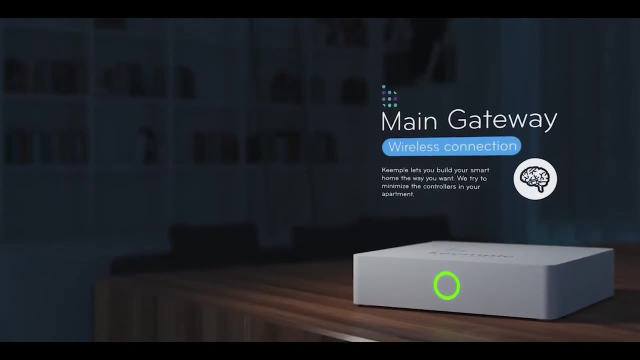 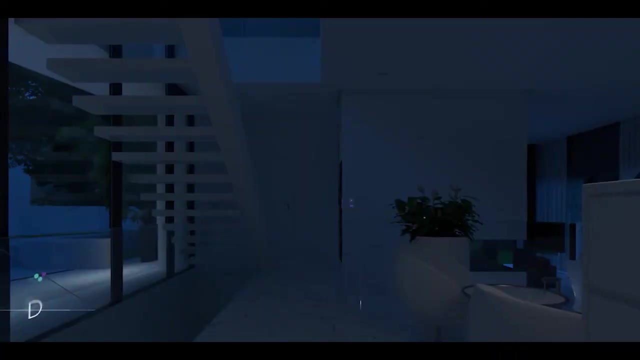 to-do lists and calendars with verbal spoken commands. Smart Homes refers to home amenities that have been fitted with communication technology enabling some degree of automation or remote control. It includes control of air conditioning, heating and lighting through voice-activated commands or mobile applications. 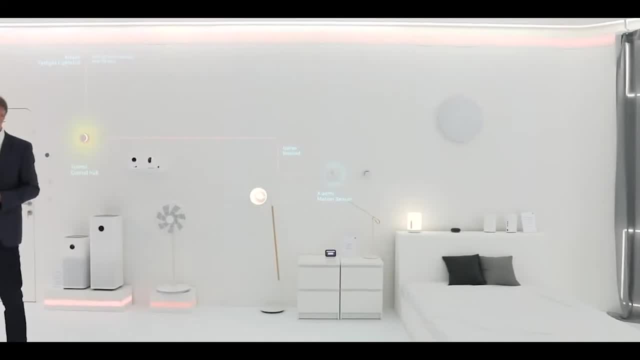 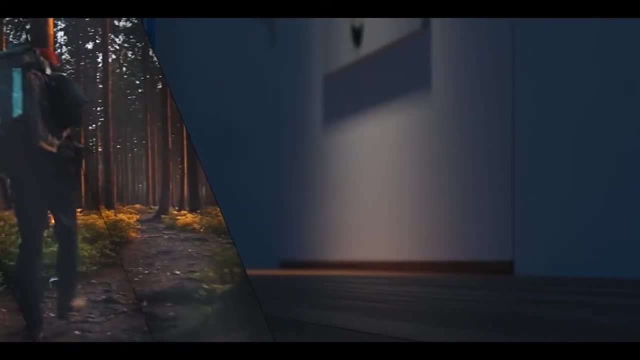 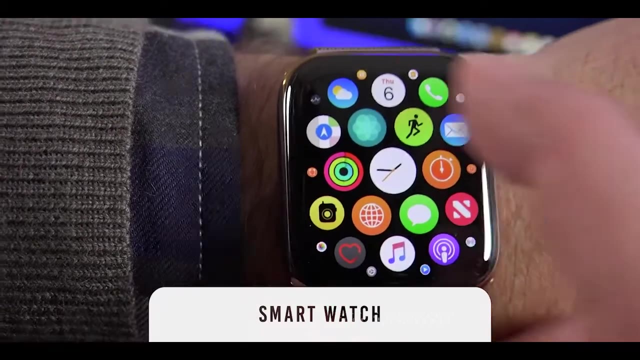 Smart Homes also include automation in appliances like fridges, washing machines and doors. Also, home security systems are also fitted with communication technology to alert the residents in case of a burglary. Accessories have become smarter as well. Smart watches are able to communicate with smartphones using wireless technology. 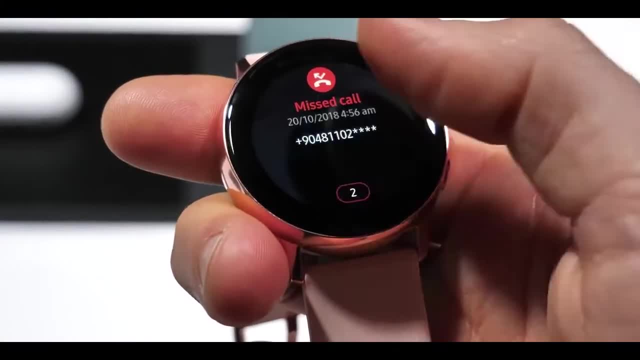 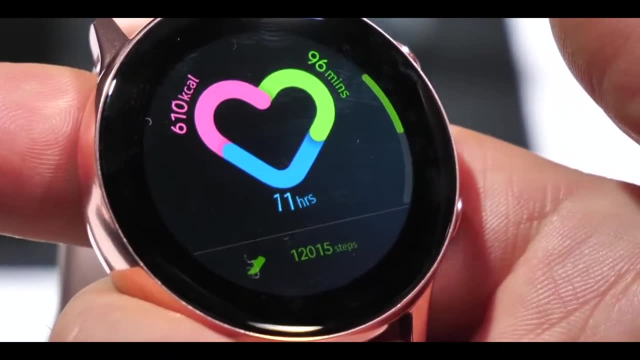 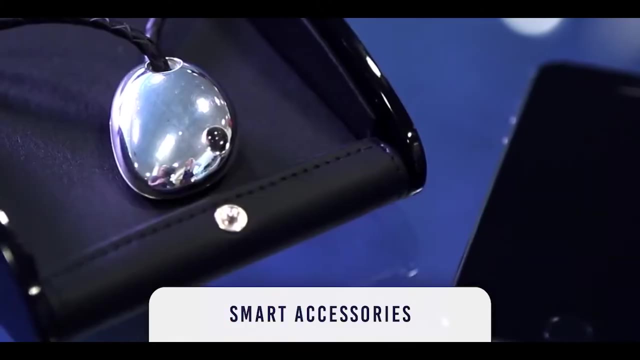 to make or receive phone calls, display messages and notifications. Smart watches can also play music, take and display photos, monitor health and fitness. run simple applications with or without a smartphone. Another smart wear device is the Cambridge Silicon Radio and Cellini Bluetooth Pendant. 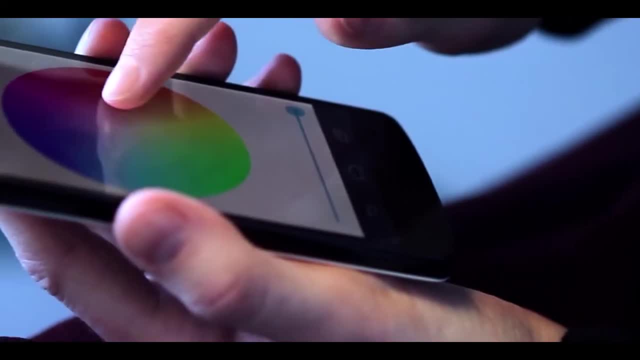 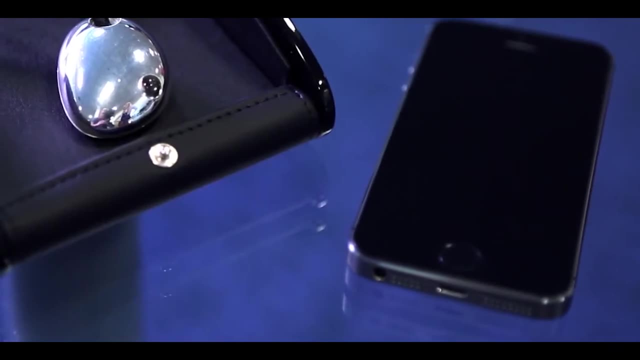 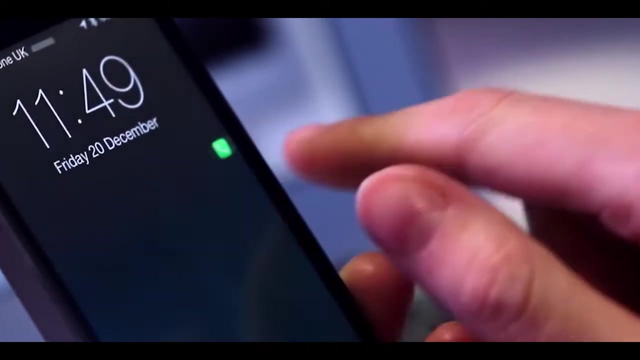 It can connect to a smartphone and is able to change its LED color or brightness depending on the mood or clothing of the user. Furthermore, it can also show notifications for the user by changing LED colors, flashing or vibrating. Another is the Smart Shoe. 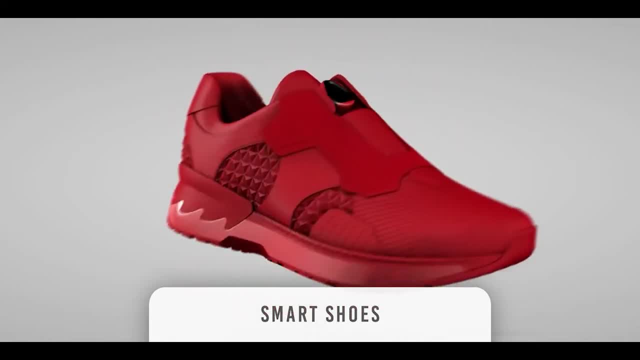 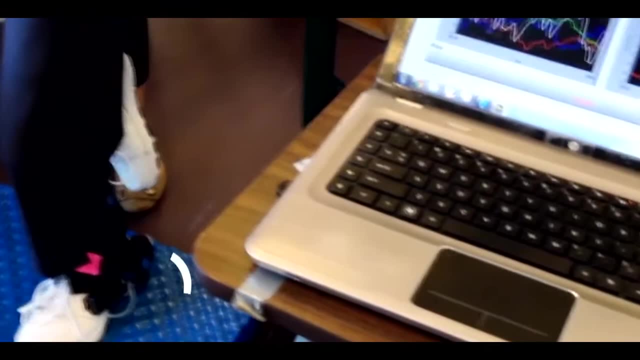 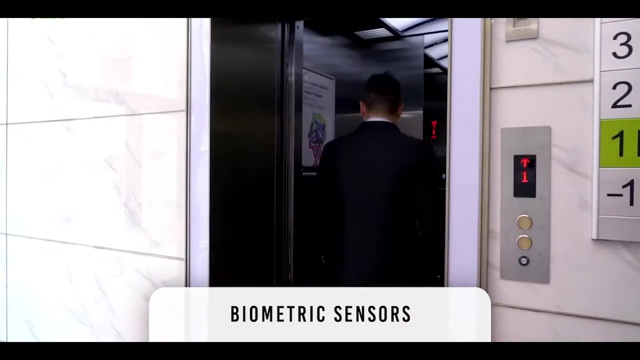 Used in their navigation and rescue operations. it is equipped with several sensors that can monitor activity levels, walking, health issues, therapy progress and give directions using vibrations. Biometric sensors are the use of human biometrics in various technological applications. For instance, biometrics can be used in access controls. 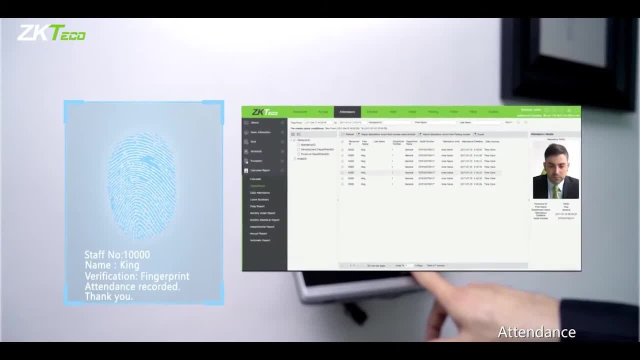 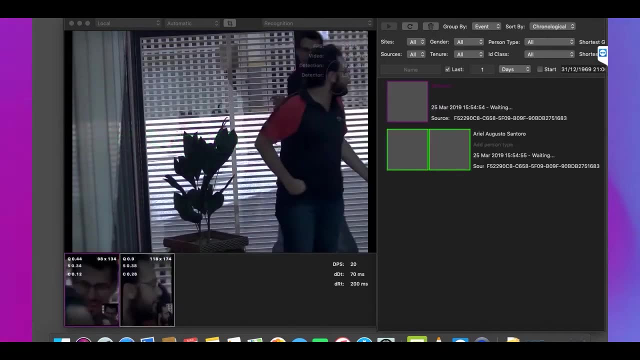 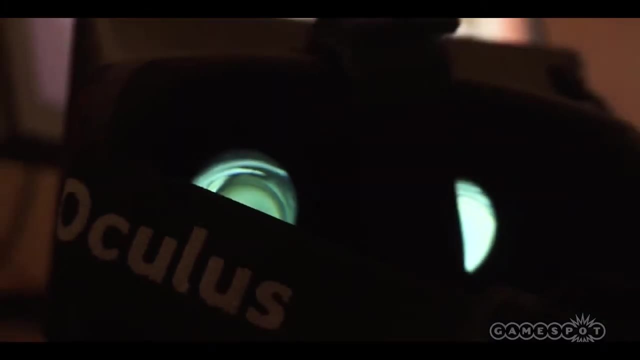 It is granting access to a computer network or security system with the use of biometric sensors. It could also be used in surveillance, for surveillance purposes by facial recognition technology. Virtual Reality, or VR, Oculuus Rift is a line of Virtual Reality headsets developed. 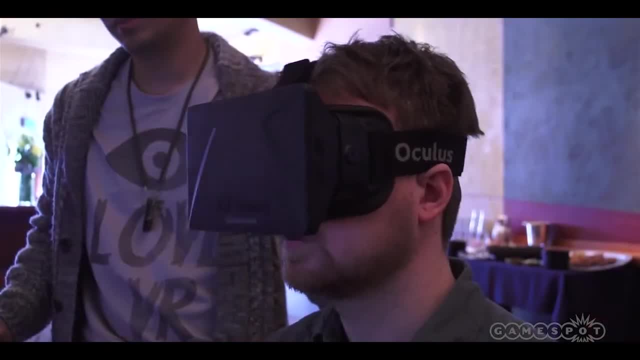 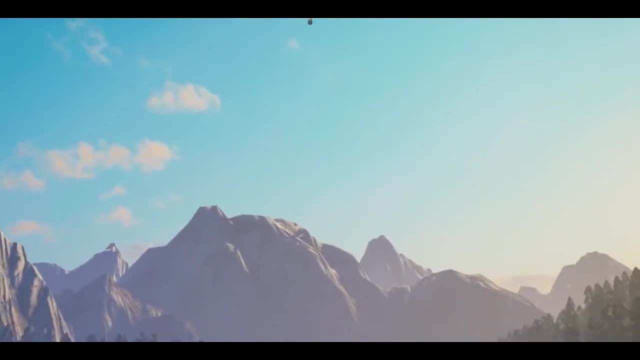 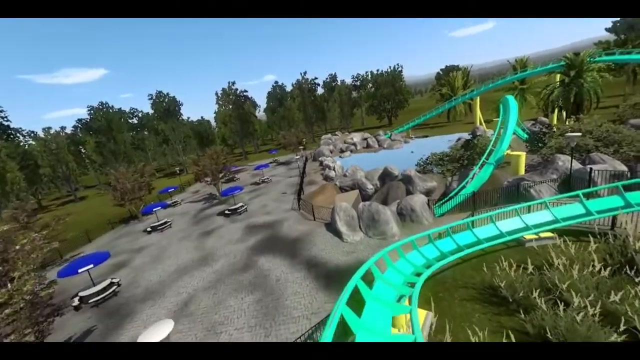 and manufactured by Oculus VR, released in 2016.. The Rift is primarily a gaming device. however, it is also capable of viewing conventional movies and videos from inside a virtual cinema environment. View new types of media like 360 degree 3D videos. 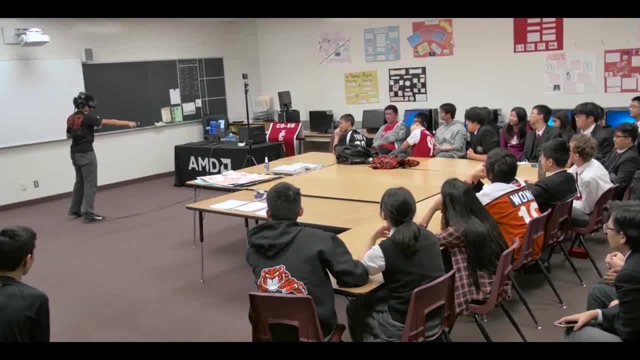 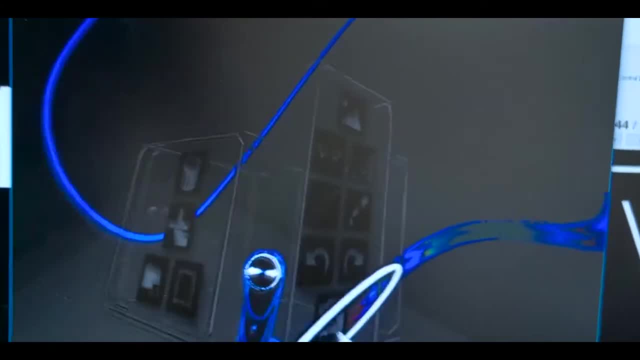 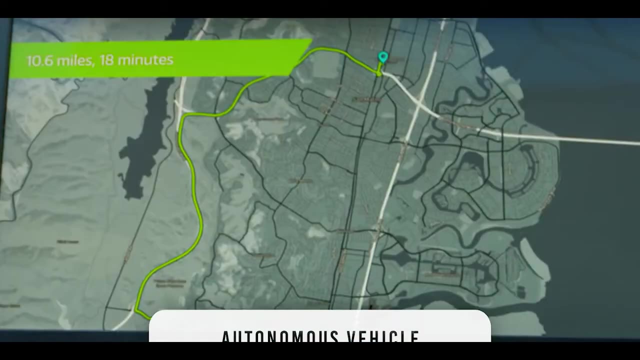 and virtual reality movies. The Oculus Rift Rift is increasingly used in universities and schools as an educational tool. It provides an immersive, engaging environment and can assist a diverse range of students for learning. An autonomous vehicle is one that can drive itself from a starting point to a predetermined. 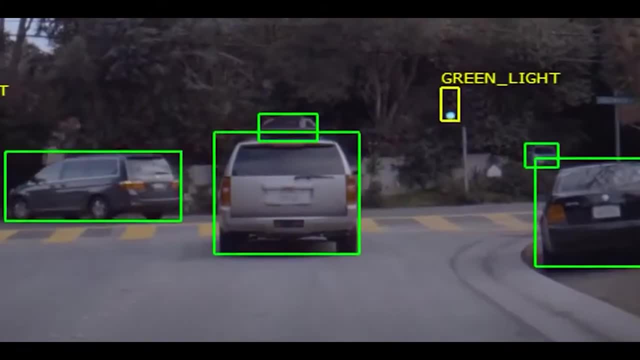 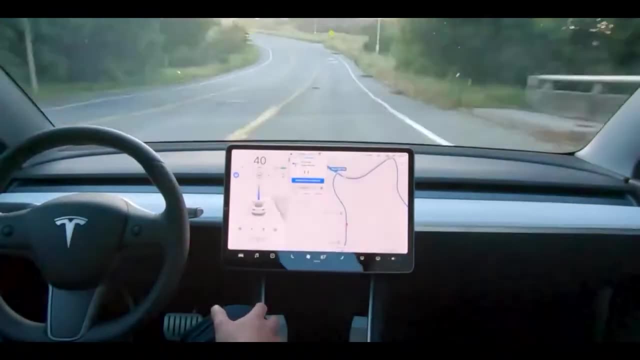 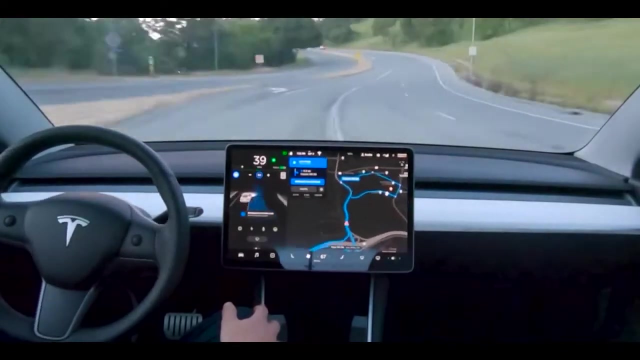 destination in autopilot mode using various in-vehicle technologies and sensors. Tesla is a company which pioneered the engineering of autonomous driving vehicles. The latest Tesla car features advanced sensor coverage, advanced autopilot technology, which allows real-time navigation updates, auto-steer technology and smart parking AI. 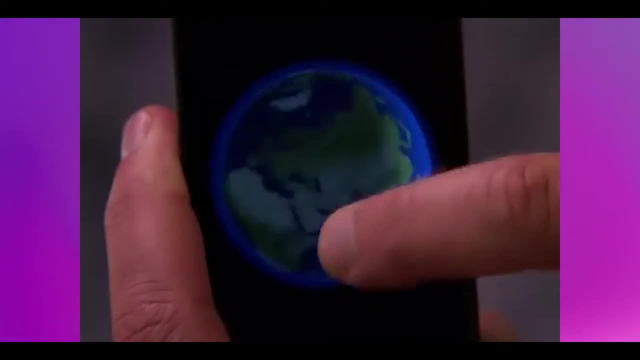 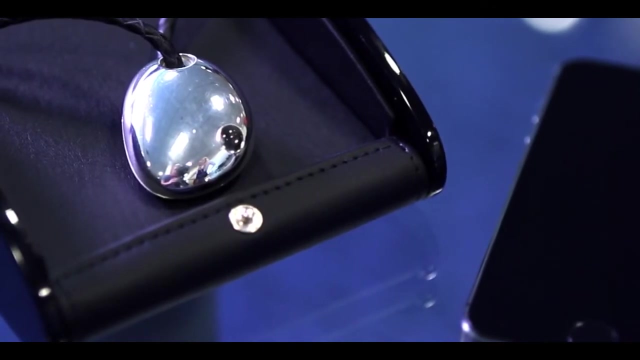 The current era of technology and HCI is indeed flourishing. It is astounding that a great leap of innovations had gone by after several decades. The present HCI is very much user-centered, more ergonomic and provide technologies to aid people with disabilities to adapt in their lives. 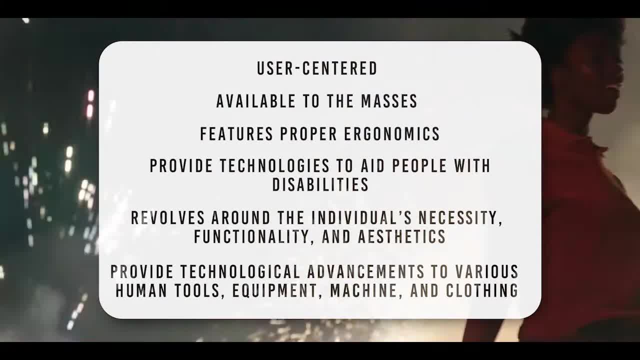 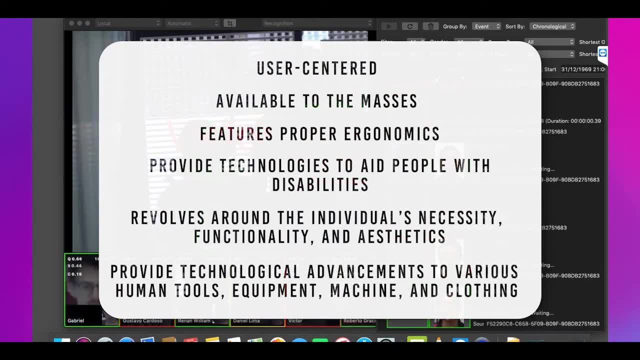 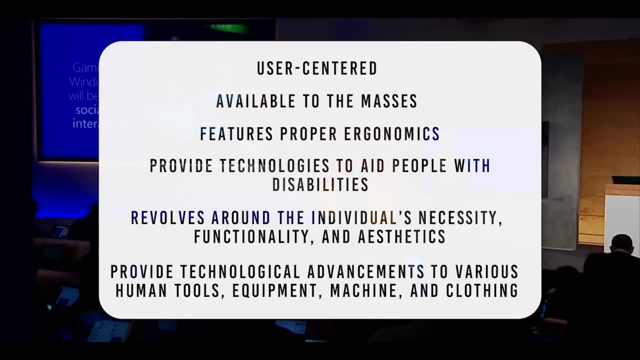 The present also revolves around the individual's necessity, functionality and aesthetics. Also, the technology is very much available to the masses and an individual who could afford to could have the privilege to own one. The present HCI is aimed to provide either technological advancements or artificial intelligence to various human tools. 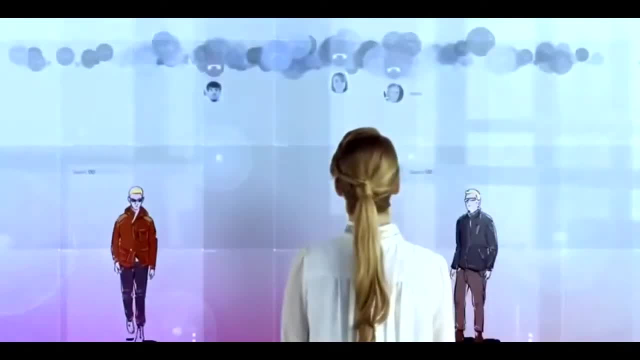 equipment, machine and clothing. What could happen to the future of our technology and the way we interact with it? Not all HCIs will be able to be developed in the future. Not all HCIs will be able to be developed in the future. 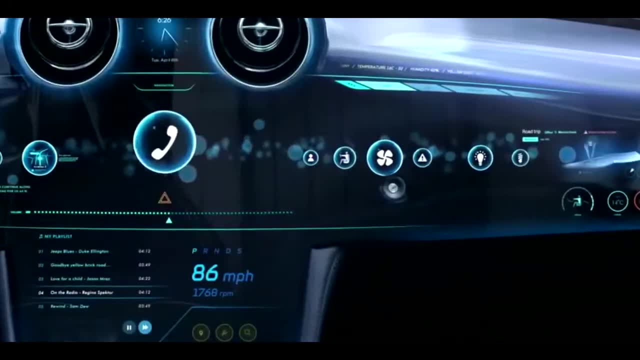 Not all HCIs will be able to be developed in the future. Not all HCIs will be developed in the future. Not all HCIs will be developed in the future. Not only our devices, but most of the things that we use in living are getting smarter every day: Our smartphones, appliances.